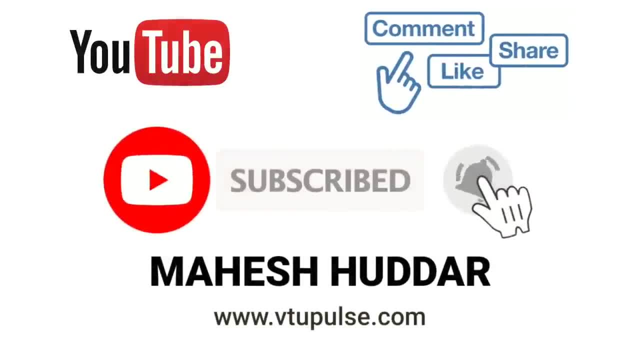 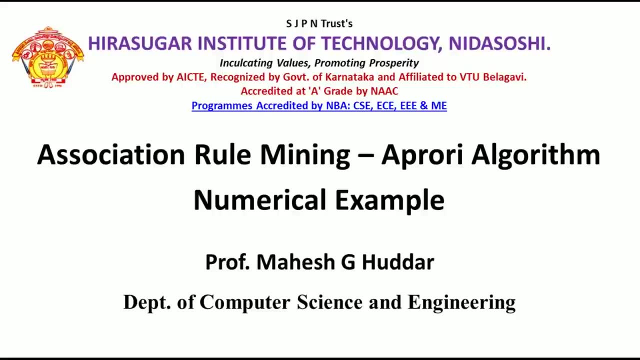 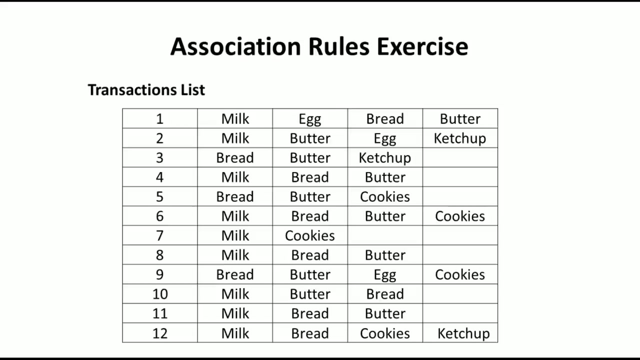 In this video I will consider a numerical example to understand a priori algorithm. It is an association rule mining algorithm. Here 12 transaction lists are given to us. In each and every transaction the different products were sold, like milk, egg, bread. 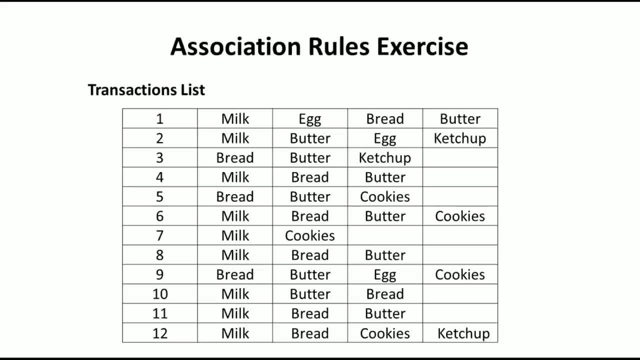 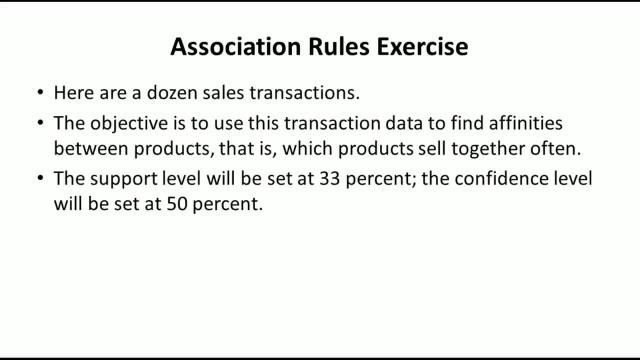 butter and so on. So what is the objective of this exercise is to identify or find the affinities between the products, that is, the products which will be sold together. That's what actually we need to identify. The support level will be. the minimum support level is. 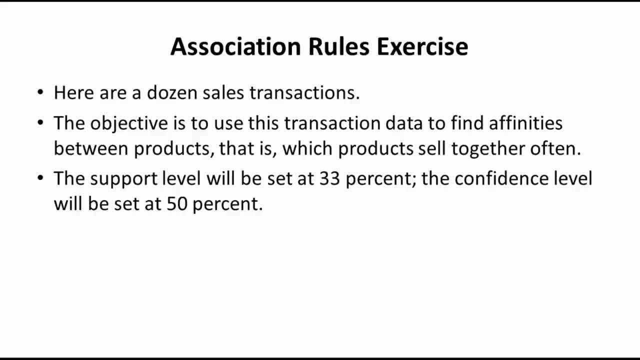 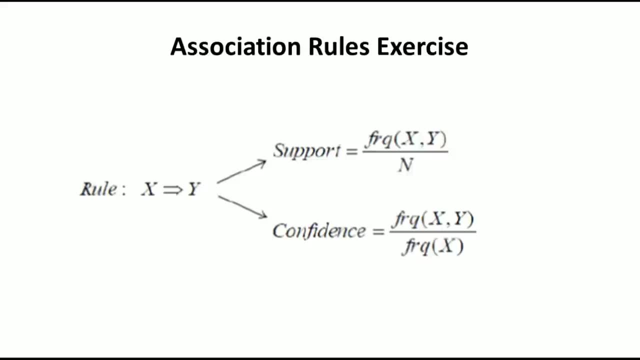 set as 33% and the confidence level is set to 50%. So that is the thing we need to do. So how to calculate the support. If you want to calculate the support for the association rule x to y, the support is always equivalent to frequency of xy divided by n. that is the 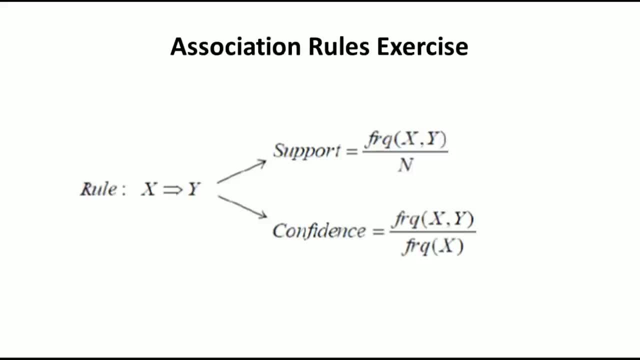 total number of transactions and the confidence of rule xy is always equivalent to frequency of xy divided by frequency of x. So this is how, actually, we used to calculate the support and confidence. So now what we need to do is we need to identify all those rules which 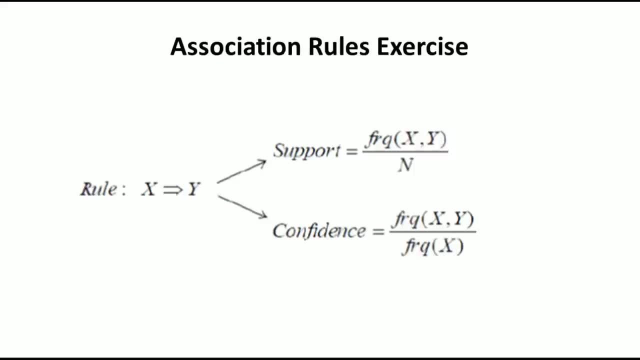 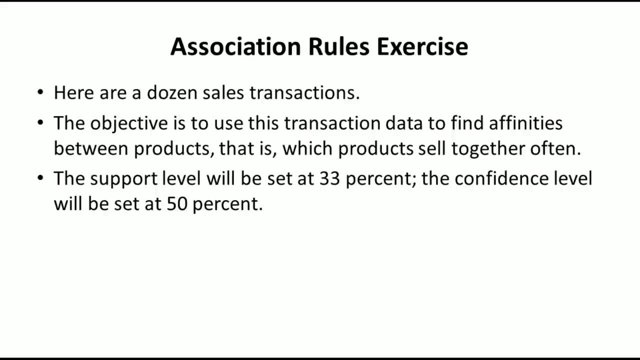 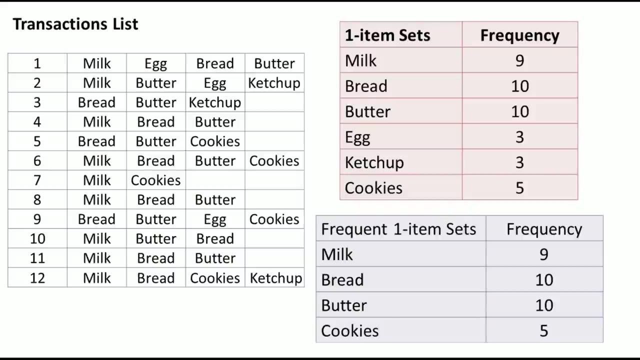 will satisfy these two requirements. So the amount of support was given 33% and the minimum confidence is given 50% in this case. So how to proceed is, first, what we need to do is we need to identify the frequent item sets and then we need to write those associating rules which will satisfy those. 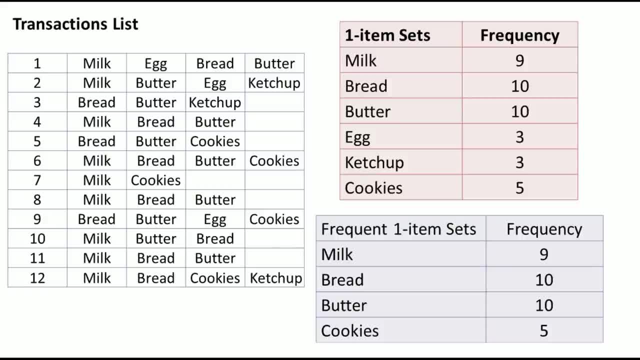 two requirements. So there are 10, 12 transactions are given to us. You can see those transactions here. First, what I do is I will create two tables. What is the first two tables I will create is I will write all the one item sets and their frequency. 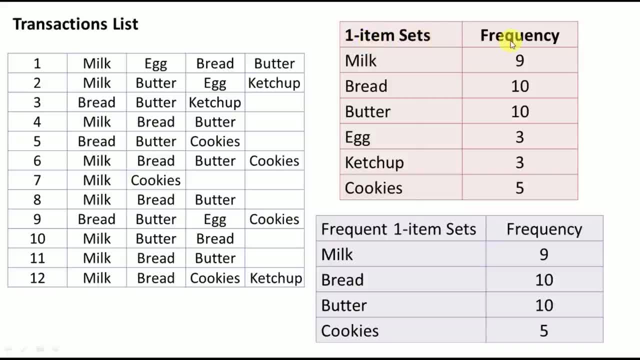 So how many items are there? There is a milk, bread, butter, egg, ketchup and cookies. These are the six products are there. Now what we need to do is we need to count how many times each product occurs. For example, how many times milk is bought out of 12 transactions. 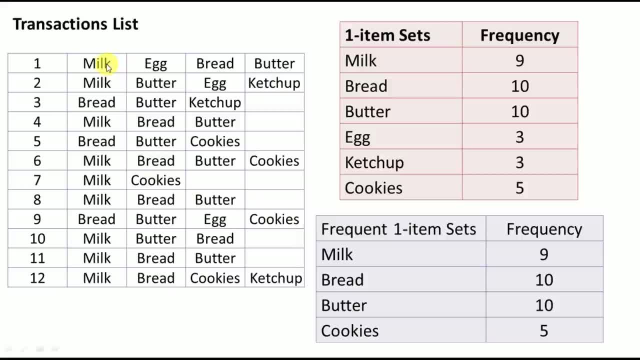 You need to just count it. So that is: in the first transaction it was bought. second transaction: it was bought. when it comes to third transaction, it is not bought. when it comes to fourth transaction, it is bought. That is 1,, 2,, 3,, 4,, 5,, 6,, 7,, 8,, 9.. So 9 times. 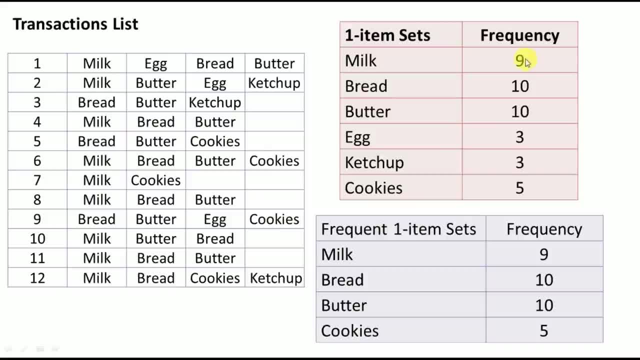 the milk was bought. So that is the one thing. we need to do it. With the same note, we need to identify how many times bread is bought. In this case, if you count it, it is 10, butter is 10, egg is 3 times, ketchup is 3 times and cookies is 5 times. So this is the first. 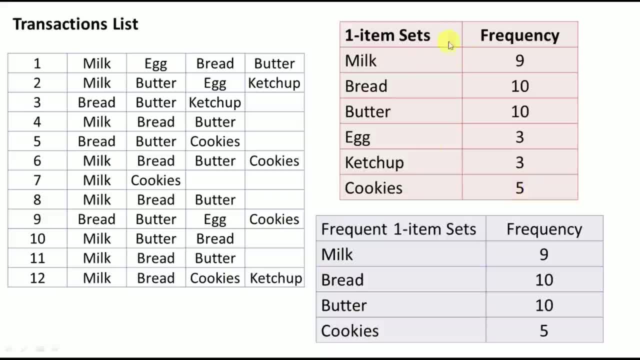 thing we need to do Now. once we do this, the next thing what we need to do is we need to create one more table Which consists of only the frequent one item sets. Here we have written all one item sets. Now we need to write frequent one item sets. What is frequent one item set? Frequent one. 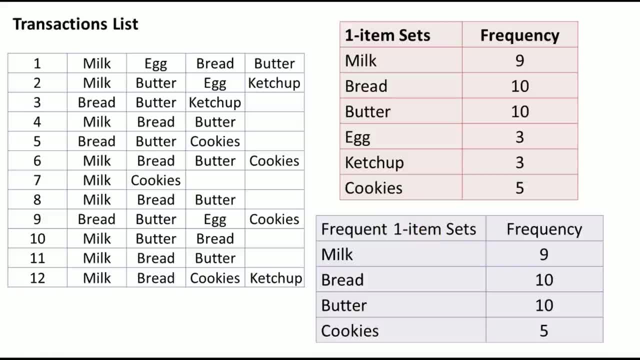 item set is the item set which satisfies the minimum support level. What is the minimum support level has been set. That is 33%. So if you want to check the 33% out of 12 transactions, if you have, for example, you can say that four transactions, assume that four transactions. 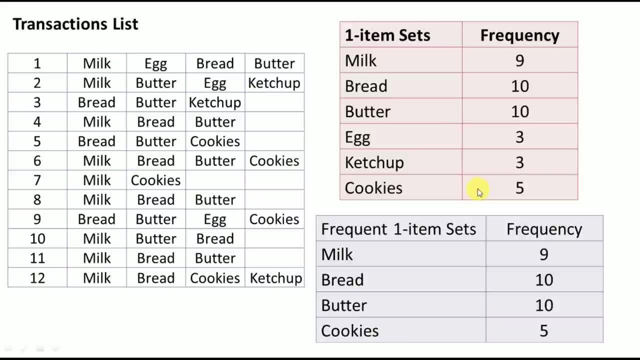 four divided by 12 is equal to how much Four divided by 12, first you need to calculate it. Just an example: I am telling you: Four divided by 12 is 33%. Okay, So what is the minimum support? we want? 30%. So minimum the particular product should be bought four. 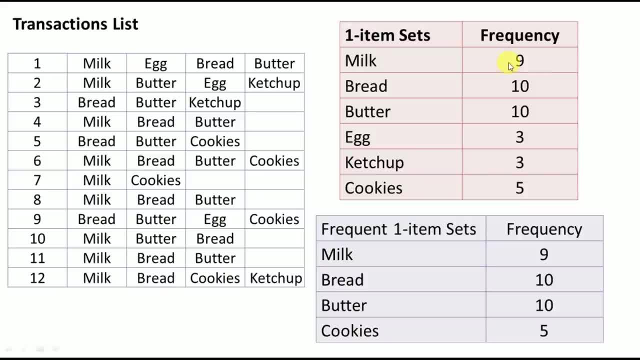 times. If it is bought for only three times, that is, a three divided by 12 is equivalent to 25%, So that is not useful for us. If it is bought four or more times, it has satisfied the minimum support Support level. So in this case, if you look at here, the egg and ketchup is bought only. 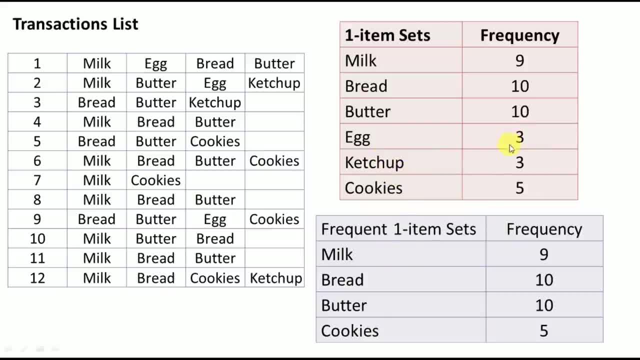 three times. So these will not satisfy the minimum support and the remaining four will satisfy the minimum support, So they will be called as frequent one item sets in this case. Now we have written the frequent item sets as well as the frequency of those things. 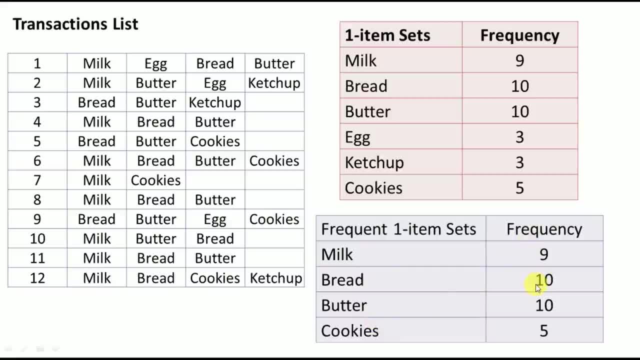 Now what we need to do is we need to write the next transaction. we need to write two item sets and then we need to calculate frequent two item sets. So that is the next thing. So how to write the two frequent item sets. These are the 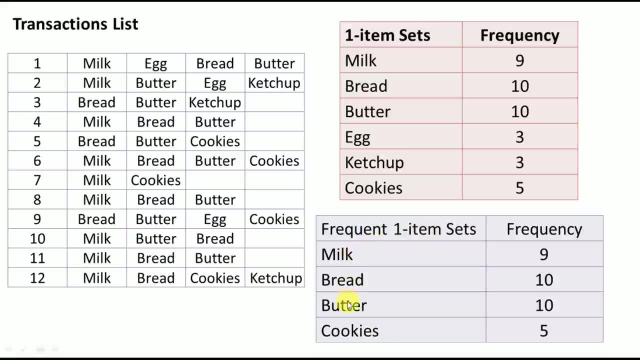 four frequent item sets. Within this we need to write the two frequent item sets, two item sets. That is the first frequent item set. two item set is milk and bread, milk, butter, milk cookies, bread, butter, bread cookies and then next one is butter cookies. So total. 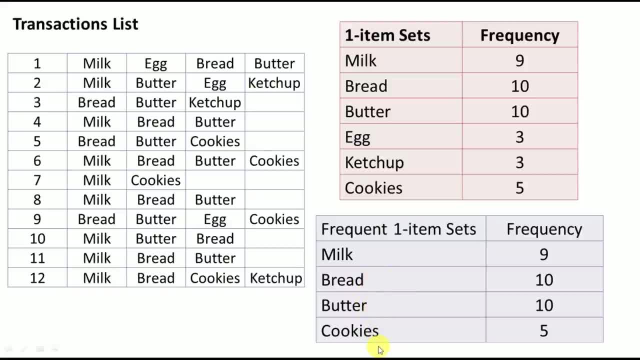 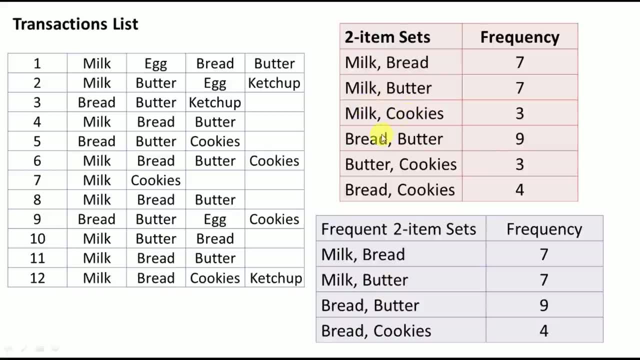 how many possibilities are there? Six possibilities. you can see those things here: milk, bread, milk, butter, milk cookies, bread, butter, milk cookies. So you can now see all the information in those. These two are the three common item: bread, cookies and butter cookies. so totally you can say that six possibilities are there. 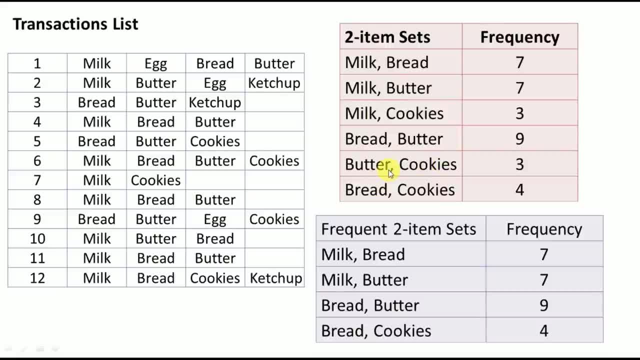 now, these are the two item sets. what we need to do here. we need to count how many number of times these two appears in 12 transactions. for example, if you go with the first transaction, milk and bread is present. the meaning of this one is the first transaction the customer has. 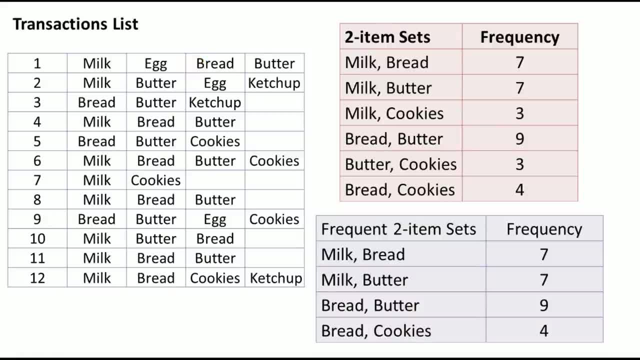 bought milk and bread together. similarly, we need to count any other place we have milk and bread. so if you go with the second transaction, we don't have third transaction, we don't have fourth one, we have milk and bread. fifth, we don't have sixth, we have seventh, we don't have, and so on. we need 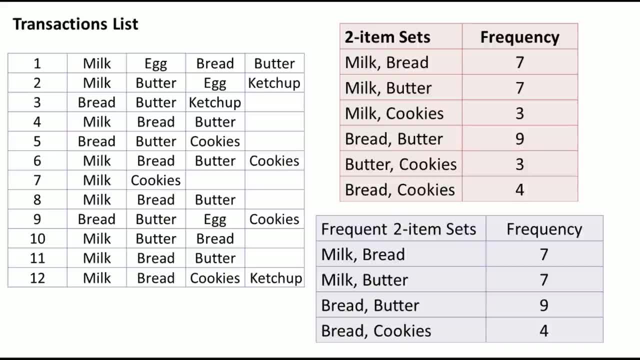 to count them. so if you count those party thing we get seven times the milk and bread is bought together. similarly milk and butter. milk and butter is present in the first one. milk and butter is present in the second one. milk and butter is present in the fourth one. sixth one is: 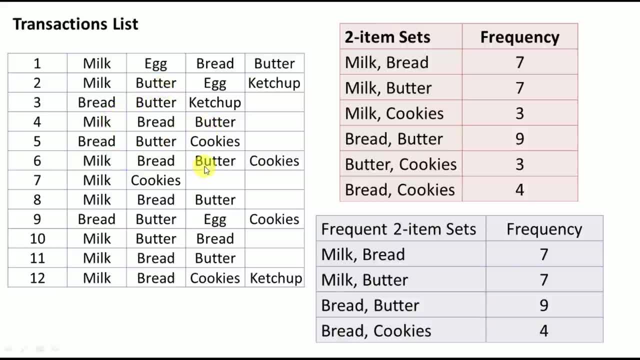 water consisting of milk and butter. eighth one is consisting of milk and butter, and so on. if you just count it, we will get seven here. similarly, we need to calculate- we can say that- how many times each of these two item sets are appearing in the 12 transactions. so this is how actually we do. 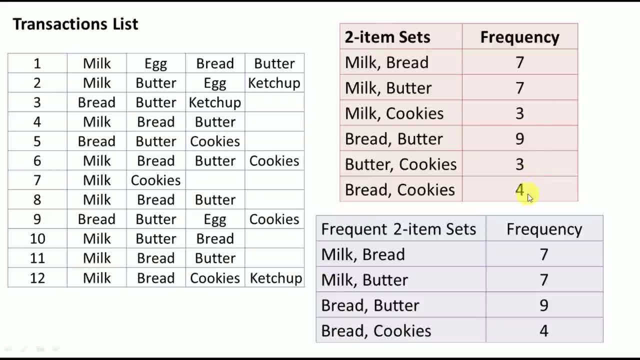 now, once we do it, we need to calculate frequent two item sets. okay, so in this case, frequent two item set. again, an item set is called as a frequent item set if it satisfies the minimum support level. so what is the minimum support level? 30 percent. if you want 30 percent minimum, it should have. 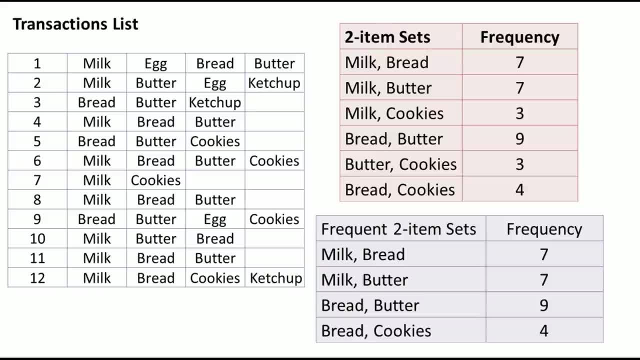 appeared four or more times. so in this case, if you look at here, milk and cookies is appearing three times, butter and cookies appearing three times. these two will not satisfy the minimum support, because the support in this case is 3 divided by 12, that is equivalent to 25 percent. 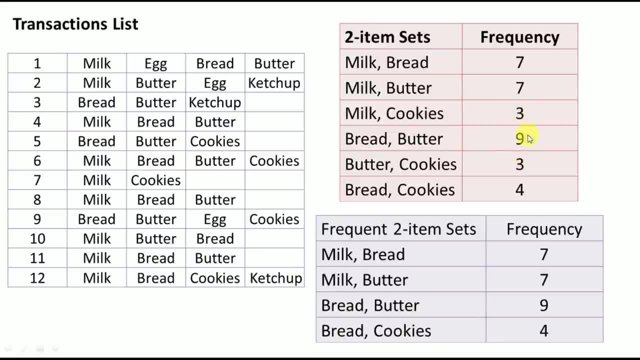 3 divided by 12, which is equivalent to 25 percent, that will not satisfy. but what about 4? 4 divided by 12 is equivalent to 33 percent. that will satisfy the minimum support. so we have only four, two frequent, two item sets, that is, milk bread seven times milk butter seven. 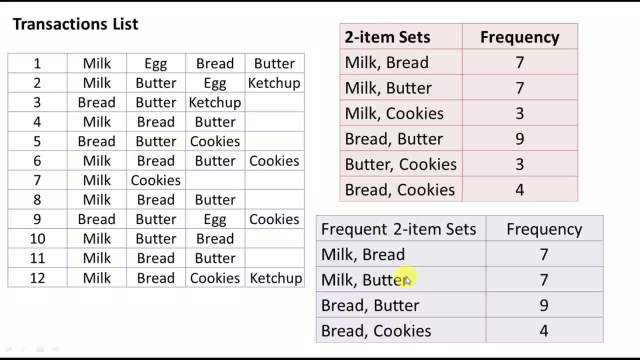 times bread butter nine times and then bread cookies four times. now what we got- frequent two item sets we got. what is the next thing we need to do? we need to calculate what is the three item sets. so what are the unique item sets? we have here items. we have here milk, bread butter and then 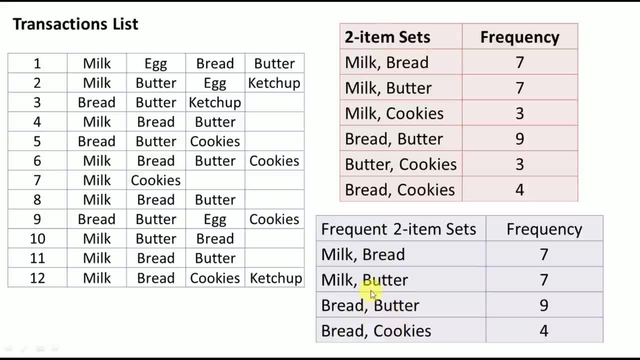 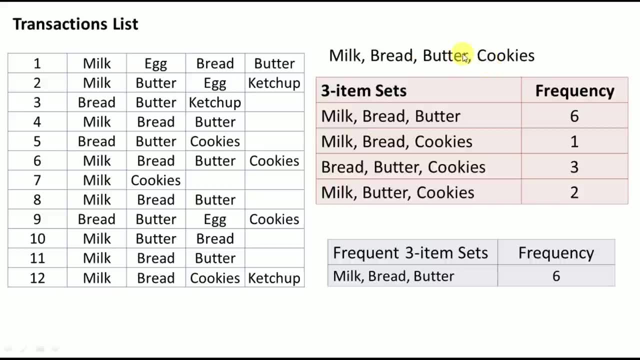 cookies. we need to find three item sets, so just check it out: milk bread butter cookies. these are four things we have. we need to write a three item set at a time. how can you write it? milk bread butter. that is the one item set. milk bread cookies. that is the one more thing. milk butter cookies. 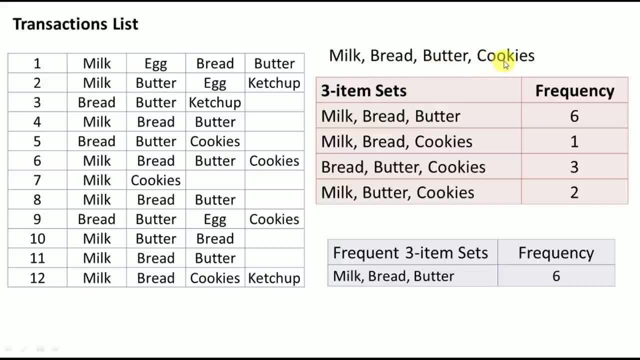 that's the third one. bread butter cookies. that is the fourth one. so that is the one I have written here. now, once you write it, what is the next thing I need to do? I need to count these three items, how many times they occur in the transaction list. milk bread butter. milk bread butter. it is. 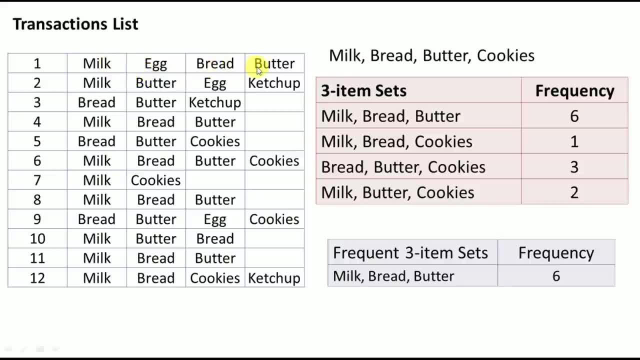 occurring here: milk bread butter, milk bread butter three times. uh, if you come to this one, uh, milk bread butter four time, milk bread butter five times, milk bread butter six time. so how many times it is appearing six times? similarly, we need to identify Milk bread cookies, milk actually bread. 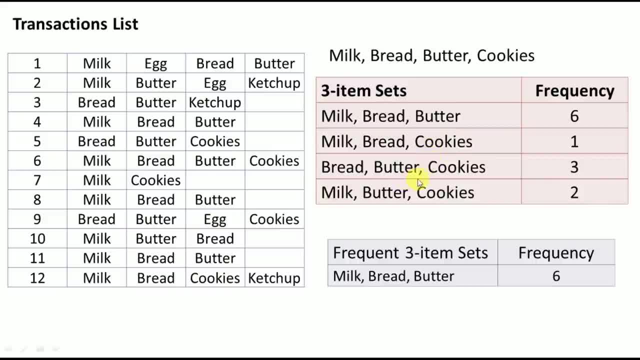 butter cookies, milk butter cookies is. so once you do this one, we got the frequency of all these three item sets. now we need to check which one will satisfy the support level, which one will satisfy the minimum support level. only the first one, because it is the frequency of milk bread batter, is 6 and remaining is 1, 2 and 3. 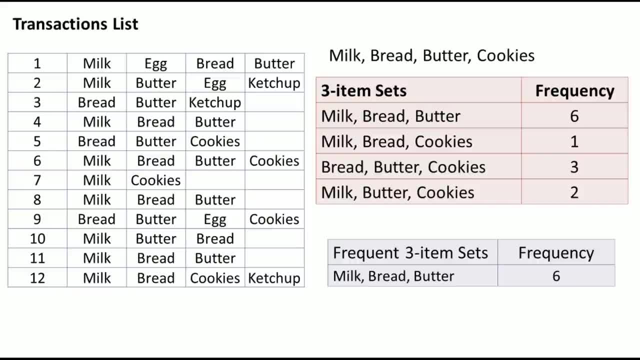 if we consider the support of these three, which will be less than the 30 percent, that is 3 divided by 12, which is equivalent to 25 percent. now, that is less than 30 percent. so definitely 1 divided by 12 and 2 divided by 12 is also less than 30 percent. now, what is the frequent three item set? 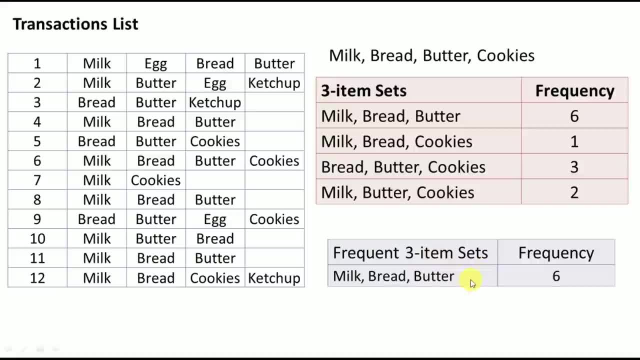 we got milk, bread and butter. what is the frequency 6 in this case? now, can i form the four item set? definitely not, because we have only three items here. it is not at all possible to form four item sets. so this is the last step step here. so what is the frequent item? 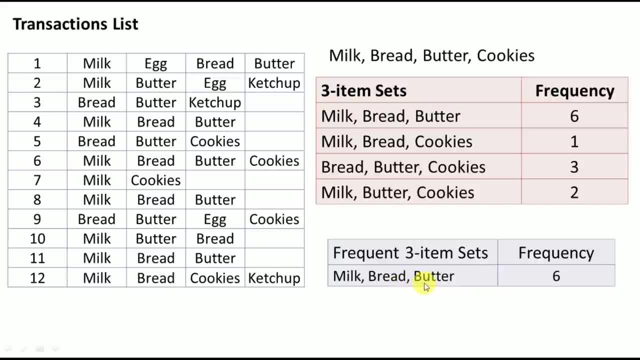 set, which is equivalent to 25 percent. that is less than 30 percent. so definitely 1 divided by 12. we got is milk, bread and butter, and it is appearing six time over here and the support of this one is 6 divided by 12. that is equivalent to 50 percent, which is more than the minimum. 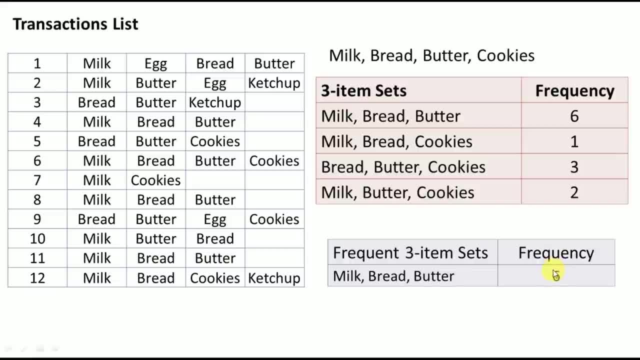 support here? what is the minimum support? that is 30 percent and it is more than that in this case. now, this is the first part of a priori algorithm is over. what is second part? we need to identify the association rules. we need to write the rules. okay, so we can write the rules, something like: 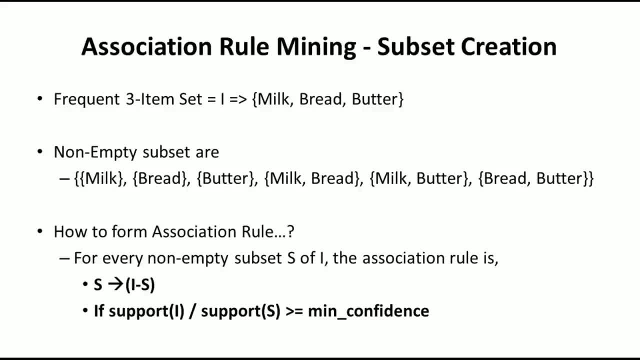 this. so, first of all, we will consider that the frequent item set is, that is, i, which is equivalent to milk, bread and butter in this case. now, if you want to write the rules, the very first thing what we need to do is we need to write all non-empty subsets of this. 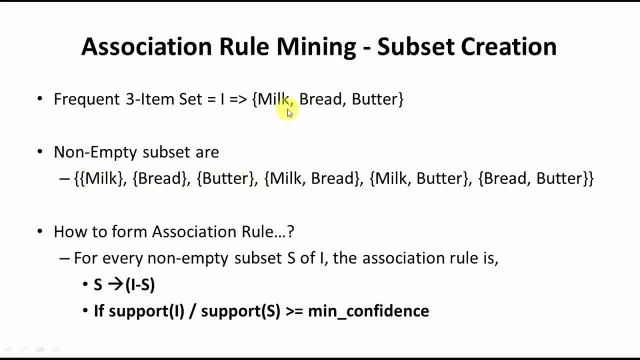 frequent item set. what are the non-empty subsets? the first one is milk, second one is bread, third one is butter, next is milk- bread, milk butter, bread butter and the last one is milk- bread- butter. that is not necessary, so we need to write all non-empty subsets of this frequent item set. 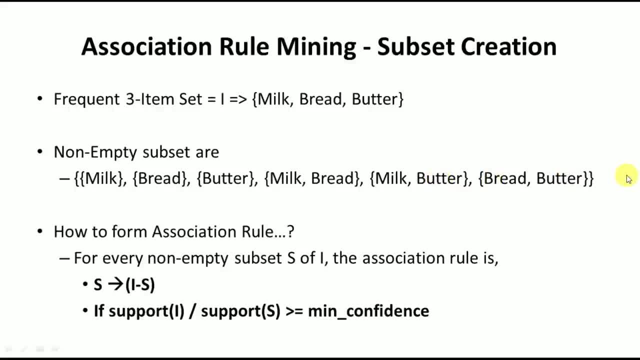 because we have that thing already here. if i use that product, there will not be anything called as a left hand side and the right hand side. so these are the non-empty subsets of this frequent item. set now how to write association rule. that's a very important thing if you want to write an. 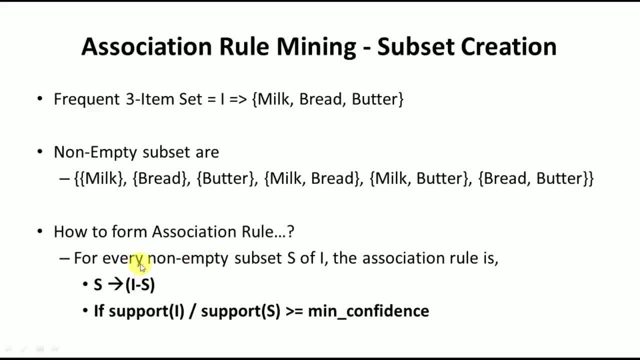 association rule. you can consider this rule for every non-empty subset, yes, of i, for every non-empty subset. these are all the non-empty subsets of i. the association rule is corn welding, a six Controller rule for well, aesthetically, 86 thing, right, if you take this one and you now you want to write non-empty subset, this is: 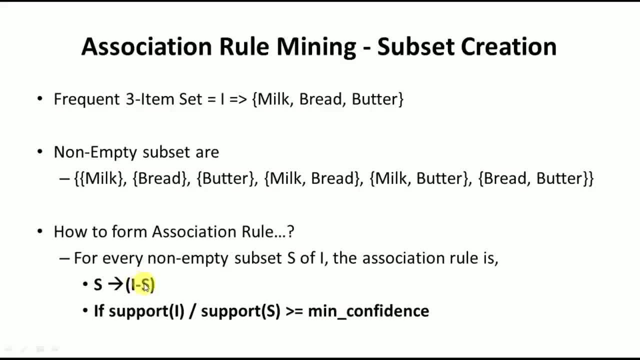 one of my favorite examples. you can write that. so let's look at it from here. you can write: yes arrow, i minus yes s is what non-empty subset. i minus s is what i is the frequent item set minus s. okay, so this is how actually we can do the reactor. so i'll take one simple example. 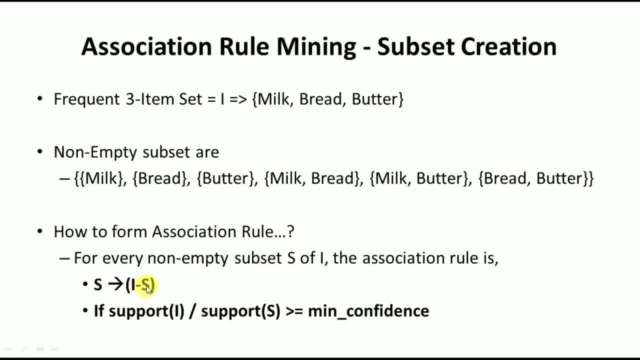 let us say that i will take s is equal to milk. that is a non-empty subset. so if yes is equivalent to milk, So that is the rule. Now we can say that this is this rule. whatever the rule we have written, it is a strong rule. If the support of I, that is, the support of frequent item. 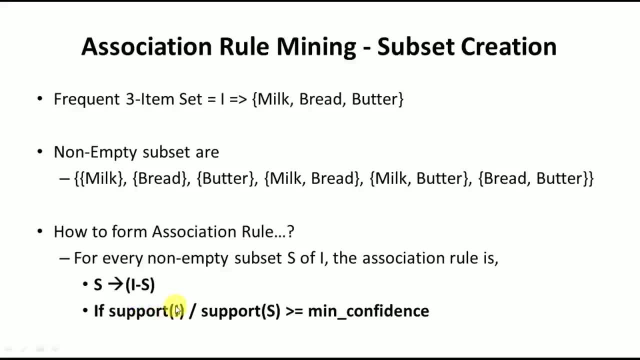 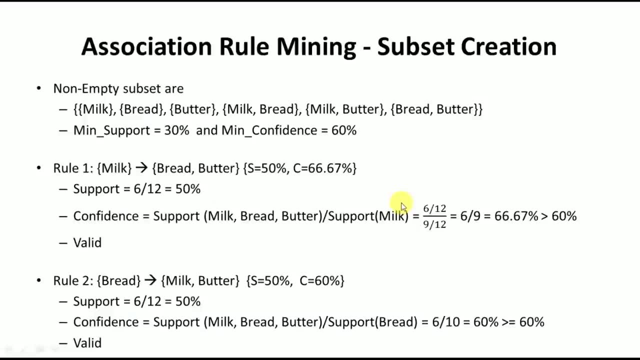 set is divided by support of, we can say that the non empty subset should be greater than or equivalent to minimum confidence. That is, support of I divided by support of S should be greater than or equivalent to minimum confidence. Okay, now we start writing the rules. First, 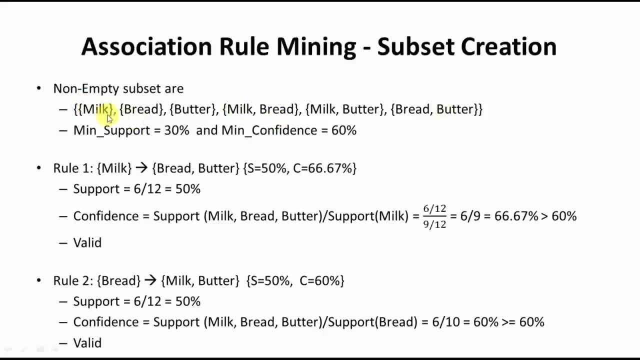 we will see this once again. that is a non empty subsets are written here. These are the non empty subset. there are six possibilities. the minimum expected support is 30% And the minimum confidence expected is 60%. So how can you write? the rule one is the rule one. 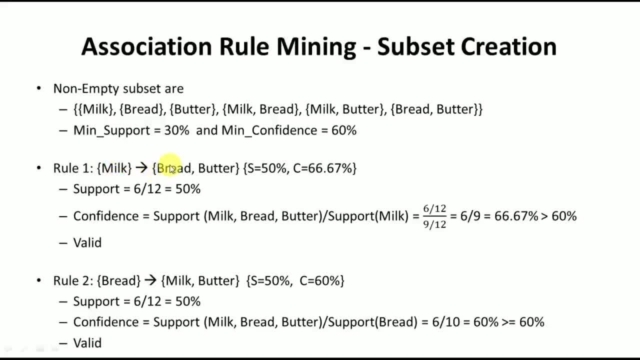 is equal to the subset, that is, S tends to I minus S. So if I consider S is equal to milk, I minus S is breaded butter. Now we need to write what is support and confidence here. So support for this particular rule is how many number of times these three are appearing, how many number of times these 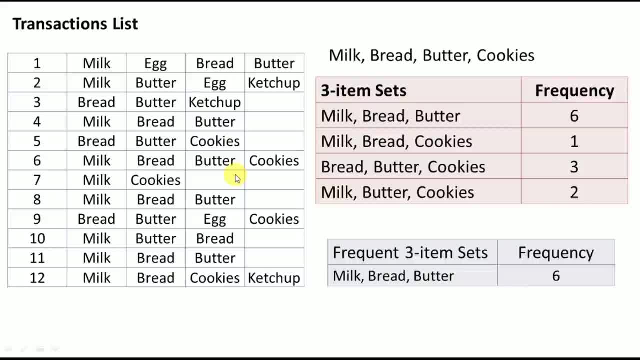 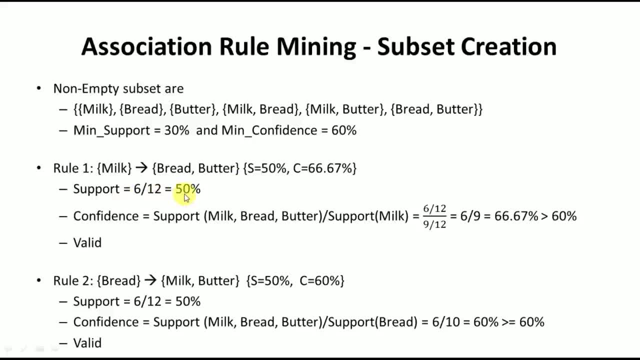 three are appearing. So if you just see this particular thing, the milk, bread, butter is appearing six times. So six divided by total number of transactions, that is 12, which is equivalent to 50% in this case. So that is what the support here. it will be same. 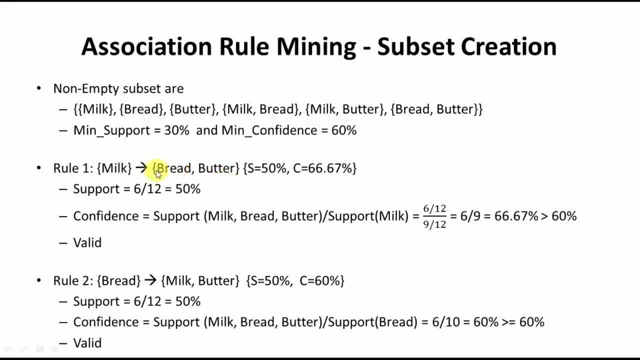 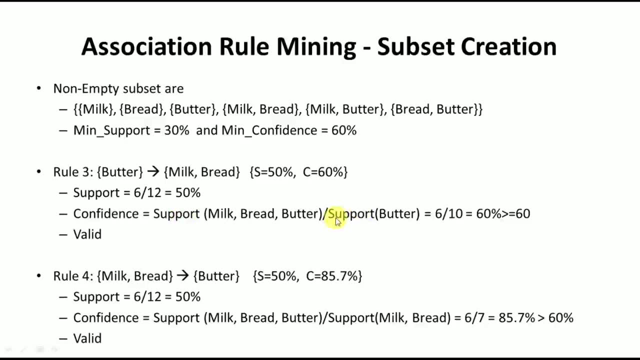 for almost all the rules in this case, because we will be considering all three while writing the rules. Now, what is confidence? we need to calculate the confidence. So confidence is always equivalent to the support of. can say that: yes, support of. I divided by support of: yes, support of. 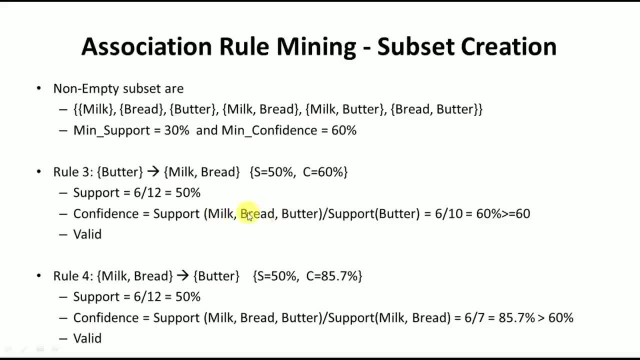 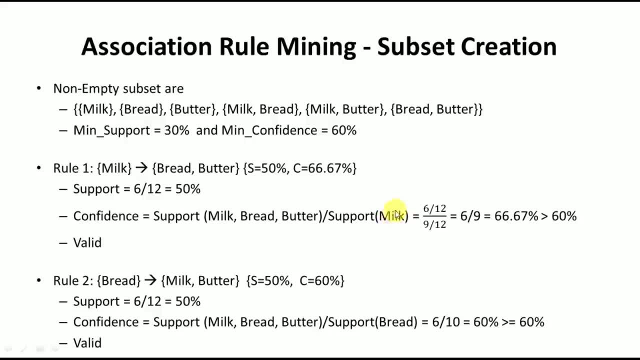 II is nothing but what? milk, bread and butter. So support of I divided by support of: yes, that is in this case the milk. Okay, so how can you calculate these things? So this can be calculated as how many number of times milk, bread, butter is appearing, as I told. 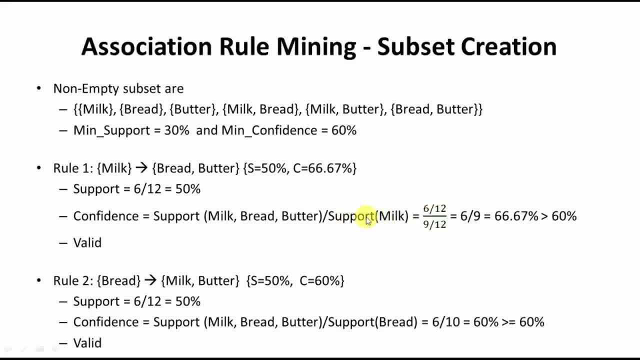 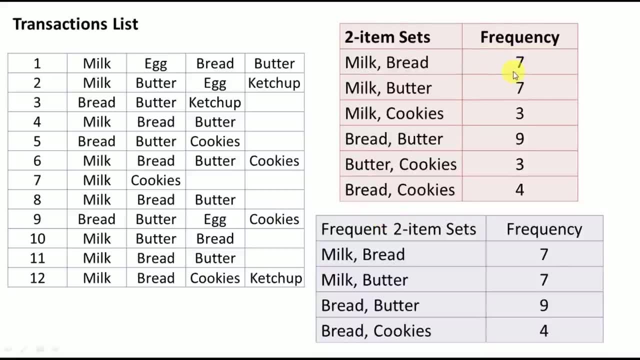 you, it is appearing six times out of 12 transactions. the milk is appearing. how many number of times? we just go back to this particular slide and then see how many number of times milk is appearing. nine times. So nine out of 12 transactions, nine divided by 12.. So 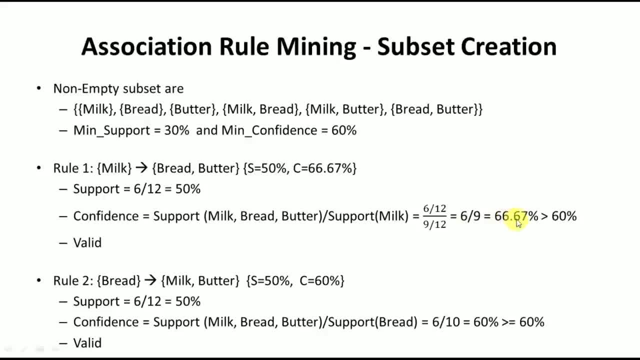 1212 will go here. six by nine will be the answer. So six by nine is equivalent to 66.67%. So it is greater than or equivalent to 60%. So this rule, whatever I have written, it's a valid rule And the confidence in this case is 66.67.. So whenever I write this particular 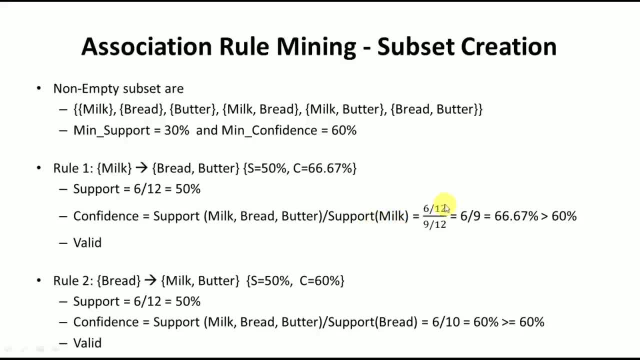 particular support of: I divided by support of: yes, this 12 will be common, So there is no need of using this one directly. we can write the number of times milk, bread butter, is appearing divided by number of times milk is appearing. that is six divided by nine. 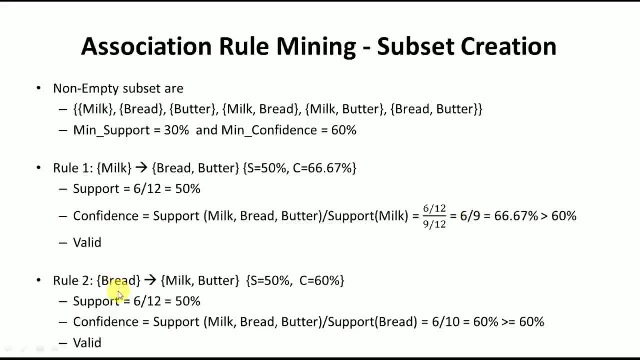 we can write it directly, Similar to this. we can write one more rule, that is, the yes will be considered as bread in this case. So what will be remaining? on the right side, milk and butter is remaining. So what is the support? as usual, it is 50%, Because milk. 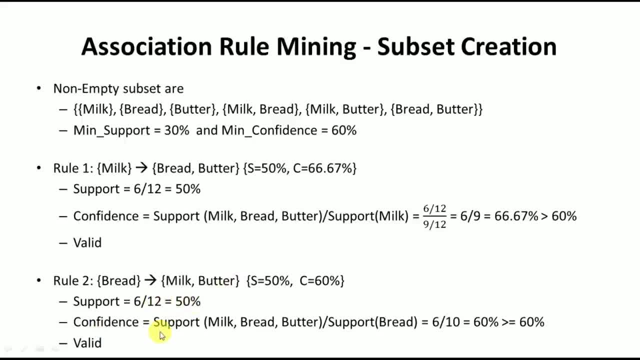 bread butter is appearing six times out of 12 transactions. Now confidence in this case. now confidence is equivalent to support of milk, bread butter. that is six. that is six divided by 12, divided by support of bread. we need to count how many number of time bread 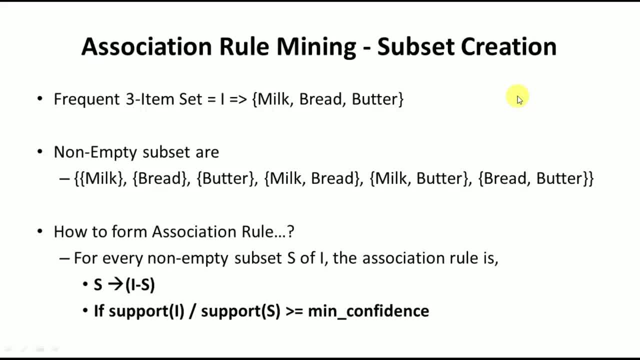 is appearing. So if you see, here it is appearing 10 times, it was 10 out of 12.. So 10 divided by 12, 1212 get cancelled. 6 divided by 12 is equivalent to 60%, which is greater than. 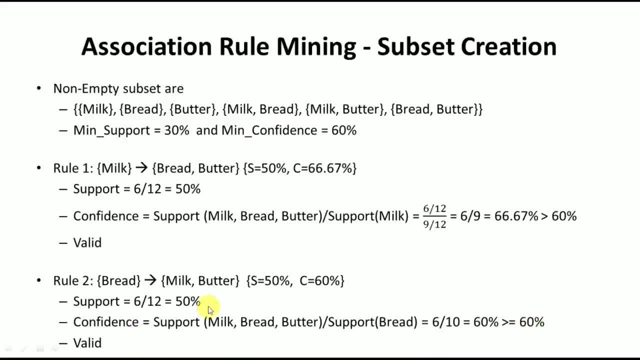 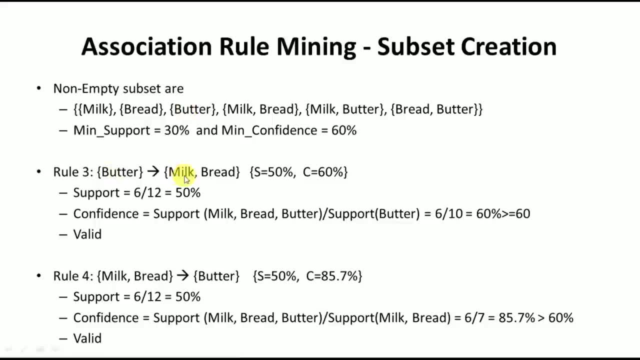 equivalent to minimum confidence. So it is again a valid rule, in this case with the confidence of 60%. Similarly, the third rule is: we will consider yes as butter, the remaining is I minus S, that is milk and bread support is again 50% When it comes to confidence. 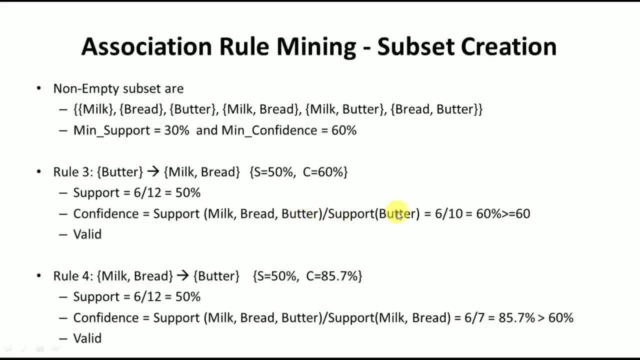 the support of milk, bread, butter is six, 12 of butter is butter is appearing, I think, 10 times. So 10 divided by 12.. That is tell it will get cancelled. six divided by 10, in this case again it is 60%, which is greater than or equal to minimum confidence, that is. 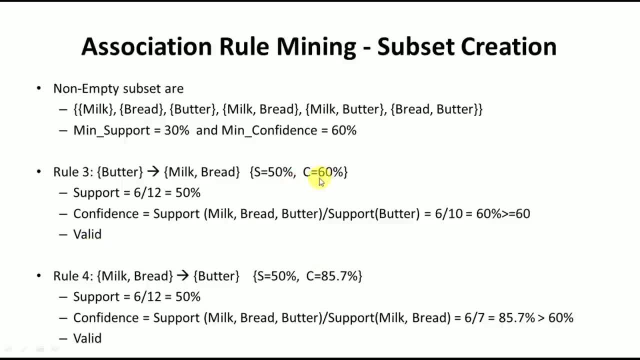 60%. So it's again a valid rule. the confidence is 60%. Now the rule number four, which is this: one milk bread will be considered as s what is remaining on the right side. butter is remaining okay. so now we need to calculate. the support is as equal as 50 percent. the confidence is. 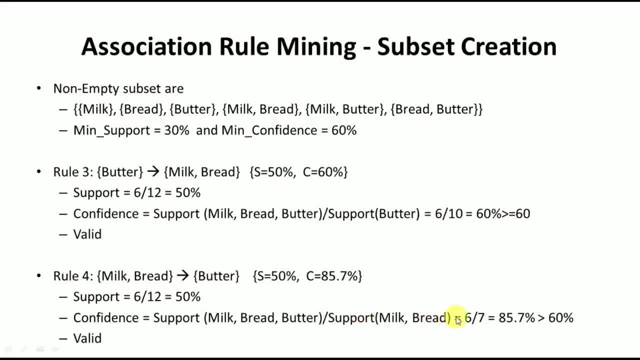 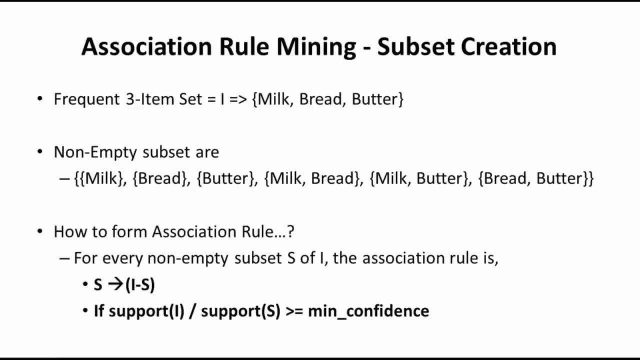 equivalent to support of milk bread butter divided by support of milk bread. that is 6 divided by 12, that is support of milk bread butter, support of milk and bread. so just go back and see milk and bread, how many times it is appearing. milk and bread is appearing 7 times 7. 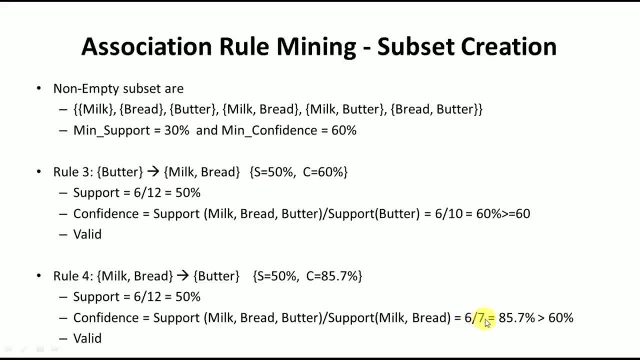 divided by 12, 12, 12 will get canceled. 6 divided by 7, that is equivalent to 85.7, which is greater than equivalent to 60. that is the minimum confidence. hence, this is also a valid rule here. now coming back to the next rule, that is milk. butter tends to. what is that? what is remaining? 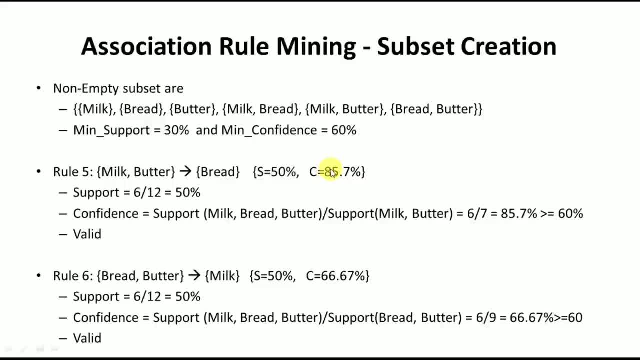 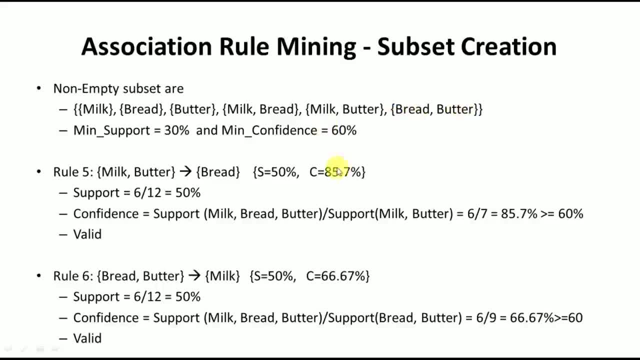 the other rule, that is, bread and butter is equivalent to S and I minus S is equivalent to milk. Support in this case is 50 percent and confidence in this case is 66.67 percent, which is again greater than equivalent to minimum confidence. Hence, this rule is also: 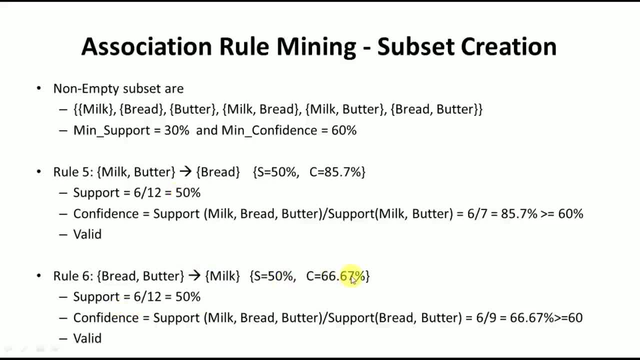 a valid rule, and the minimum confidence in this case is 66.67.. So this is how actually we can use a priori algorithm to come up with the valid or strong association rules. First we need to calculate the frequent item sets and then we need to find the strong rules.